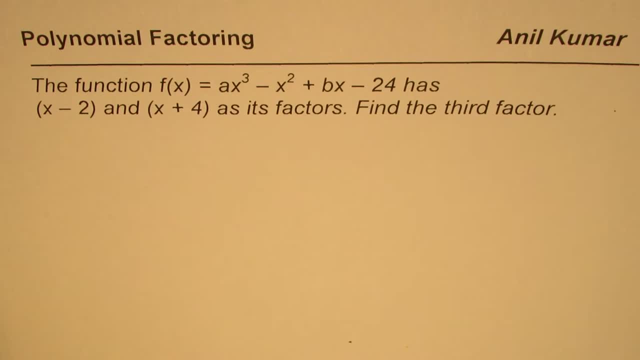 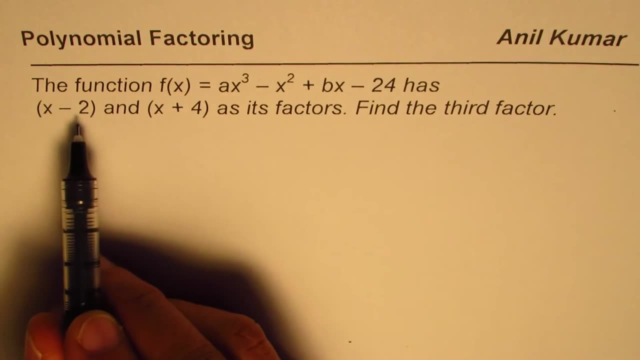 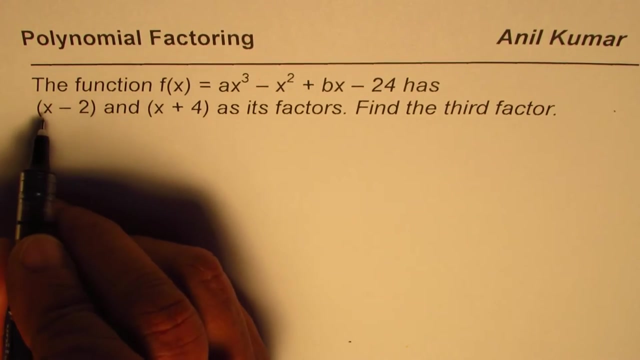 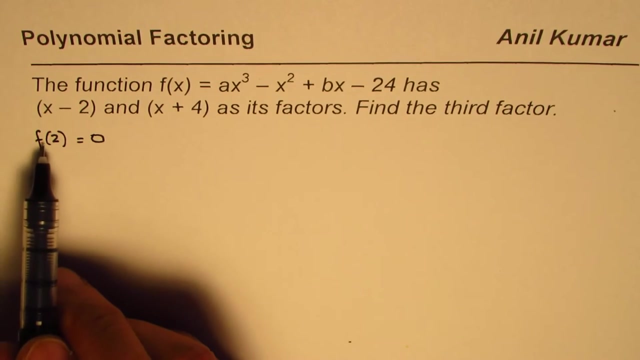 and apply remainder theorem to find the solution. Okay, so here is my solution. When we say that x minus 2 and x plus 4 are the factors, it really means let's start with x minus 2.. So if x minus 2 is a factor, that means f of 2 should be equal to 0, right? So what is f of 2?? So let me write down x as 2 here. 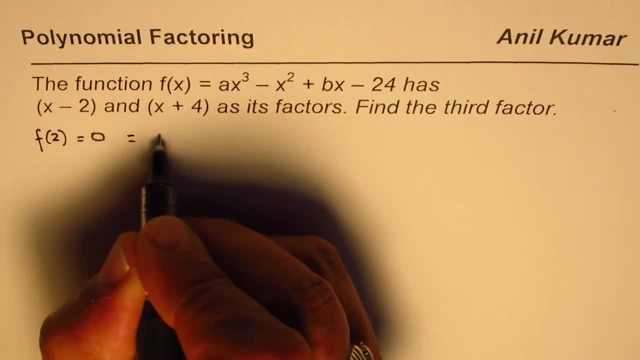 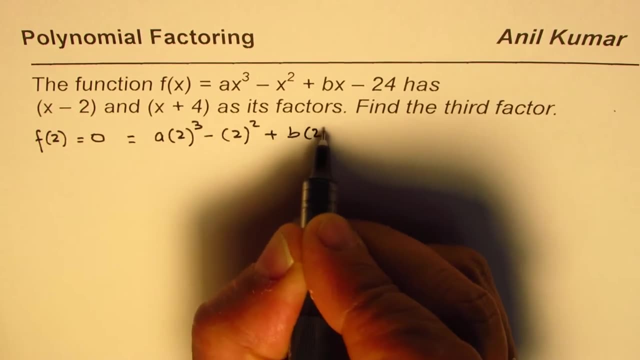 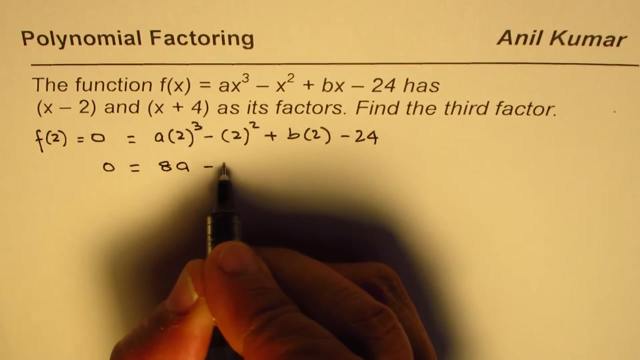 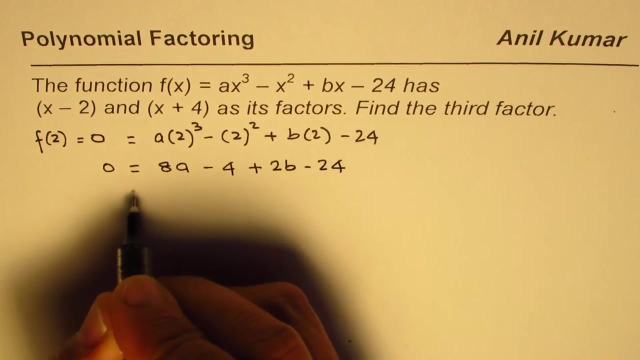 So when I write x as 2, we get a times 2 cubed minus 2, squared plus b times 2 minus 24.. So we get 0 equals to 8a minus 4 plus 2b minus 24.. We can simplify it a bit more Combining these terms: we get 8a. 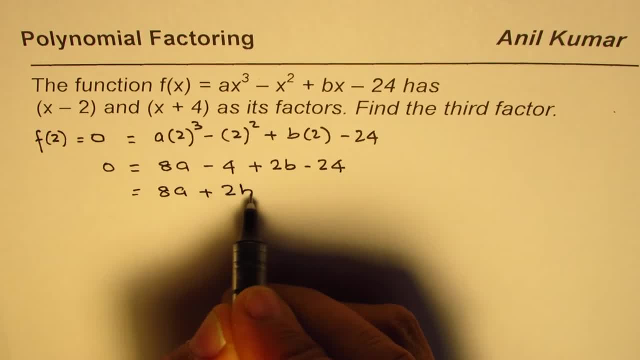 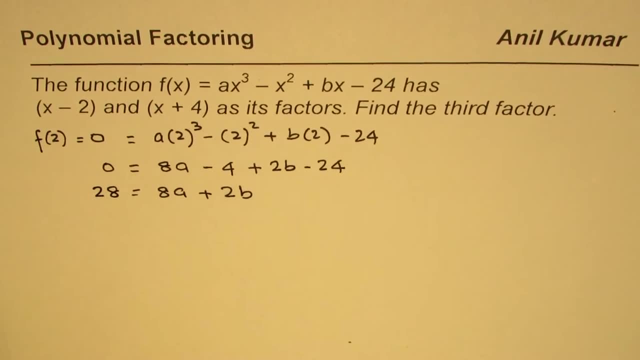 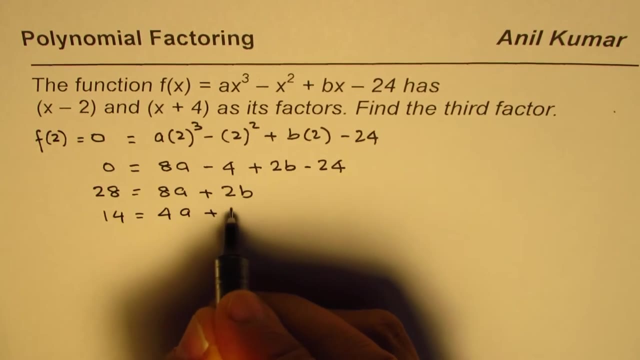 plus 2b minus 24 minus 4 is minus 28.. Bringing it to the left gives us plus 28,. right Now we can divide this by 2, to simplify, So we get 14 equals to 4a plus b, correct? So basically, we are given a polynomial cubic in two variables, a and b, To find the third factor. we need to find the. 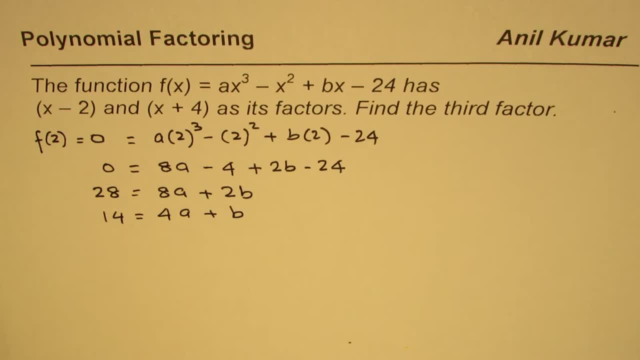 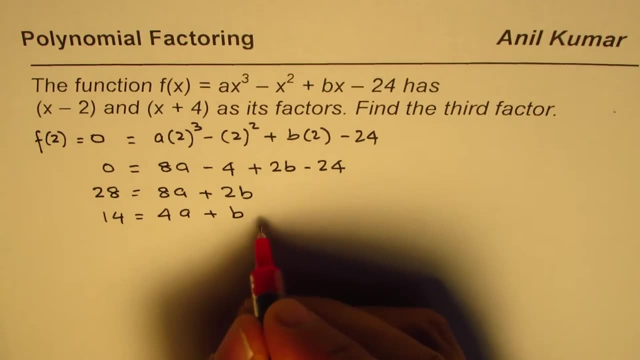 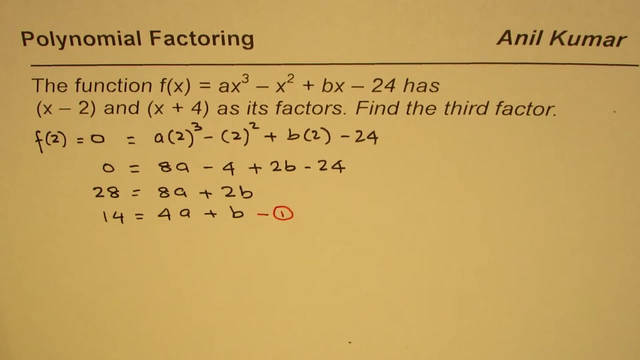 value of both a and b, and only then we can get the answer. When I substitute it to in this particular equation, I got one equation in these two variables. Let me number this equation as 1.. So I'll do the same thing with the second factor to get the second equation correct. That's the whole idea. So we can write f of minus 4.. That should be also equals to 0. Substituting minus 4 will give us this equation right. So it is minus 4.. 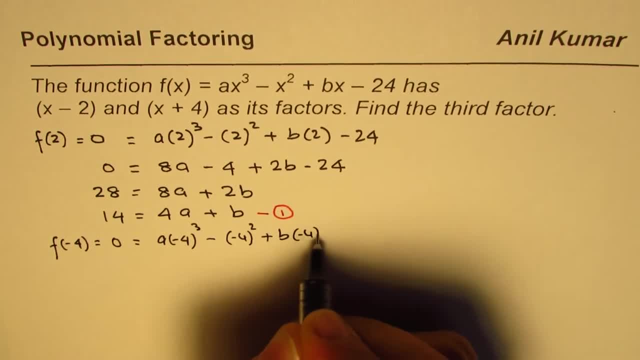 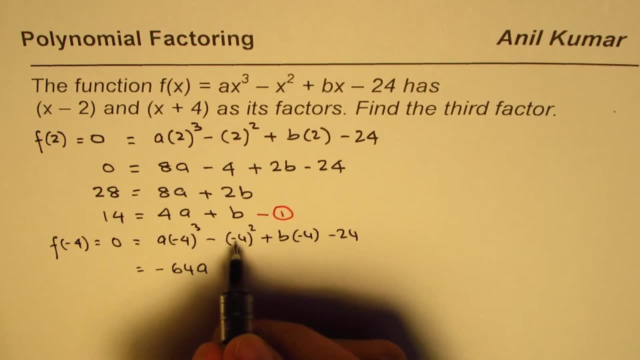 minus 4 squared plus b, times minus 4 minus 24.. This is minus 64a. This becomes plus, but with minus it is negative 16. Here we have minus 4b minus 24.. Now again we can combine a's and b. I mean rewrite this as minus 64a minus 4b. Combine these two terms. 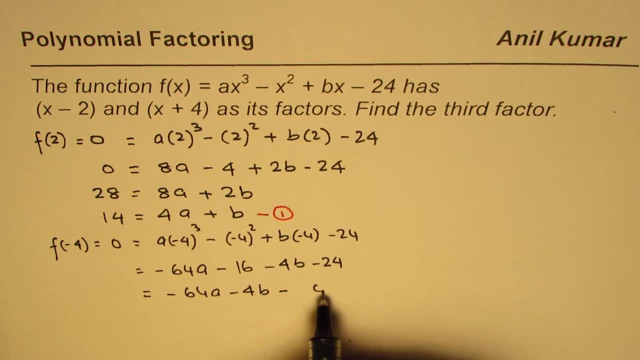 Which is negative. 6 and 4 is 10, 2, 1, 3, and 1, 4, correct. So we can actually divide all this by 4, right? So let me rewrite this after dividing by 4 and bringing minus 40 to the left side, Or let me do it in two steps. So this is all: 0. equals to correct When I bring 40,. well, these are negative, so I prefer to bring these two on the left side, So we'll write this as 60 minus. 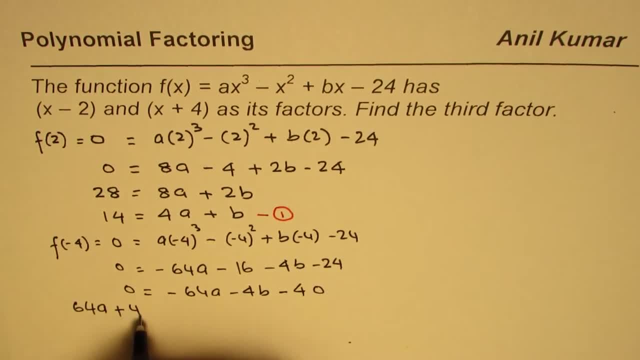 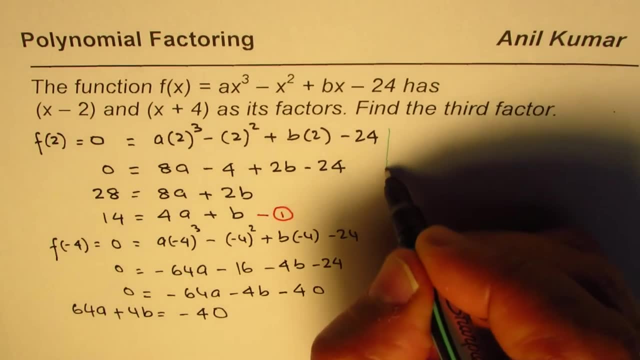 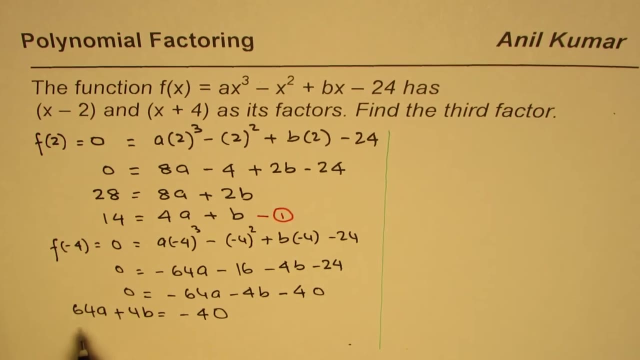 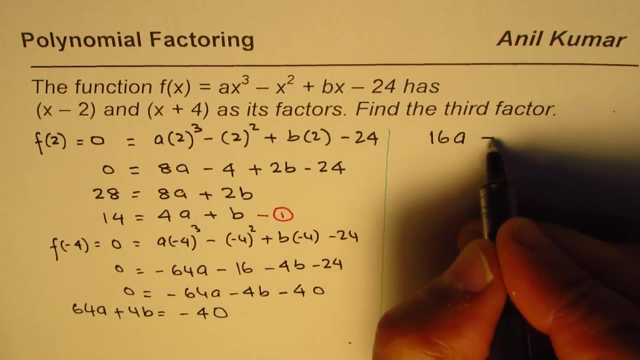 64a plus 4b equals to minus 40, correct? Anyway, let me write them on the right side, since I'm running out of space on this page, So rewrite this: dividing all these terms by 4.. So when I divide 64a by 4, I get 16a, 4b by 4, I get b, And then we have equal to minus 10.. So I'm calling this as. 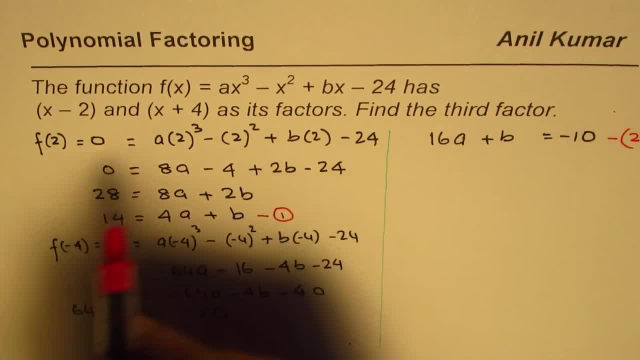 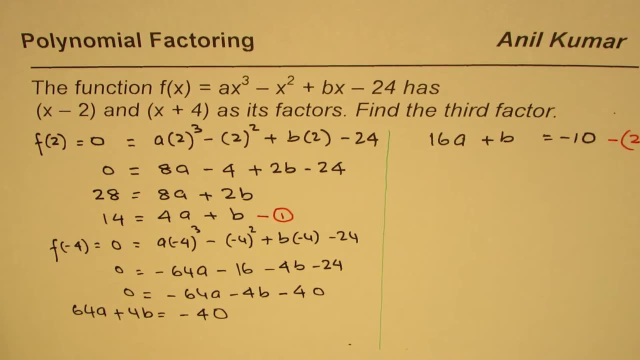 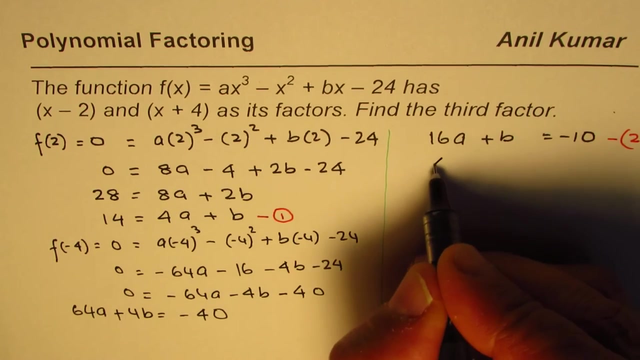 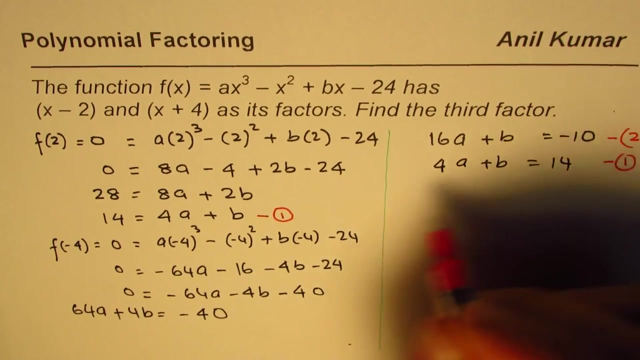 my equation number 2, okay, So these two factors help us to get two equations in a and b. Now we can find these coefficients by substitution or elimination method, right? So let me rewrite equation number 1 here itself, which is: 4a plus b equals to 14.. That is, I just copied equation number 1, right? So this I copied from here. Okay, fine, So we can easily eliminate b. 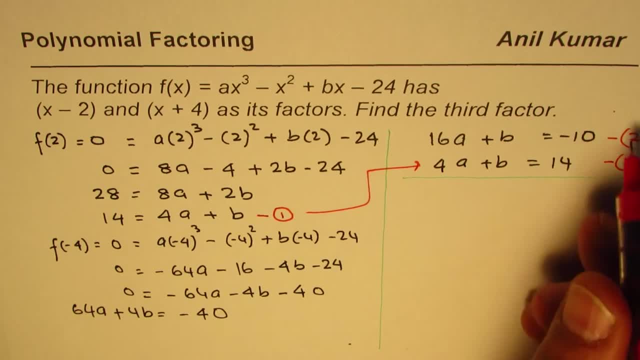 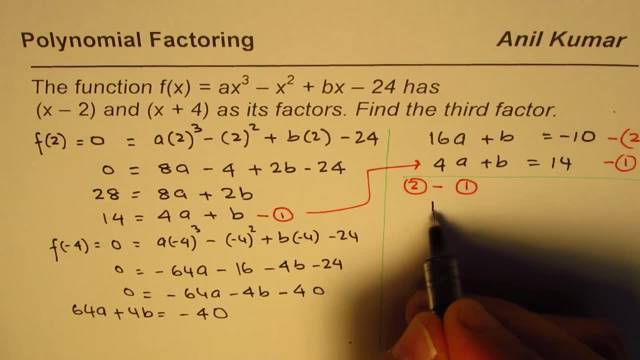 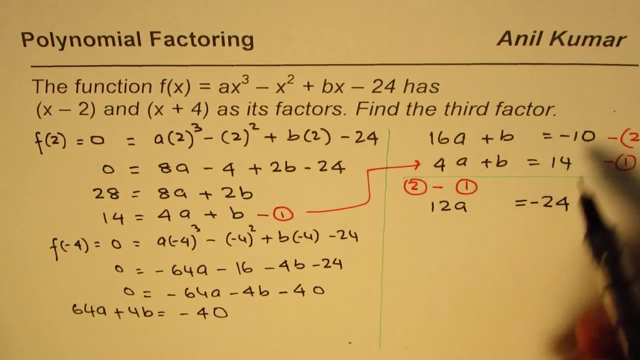 So we can eliminate b by taking away one from the other. So equation 2 minus equation 1 is what we are going to do now. So that gives us 12a. this is 0, equals to 24 with a negative sign, right, Minus 10, minus 14.. Or a is equals to minus 24 divided by 12.. And that is equal to 2 with a negative sign, So minus 2.. 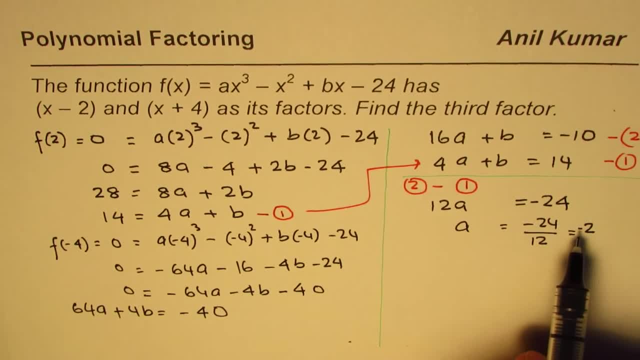 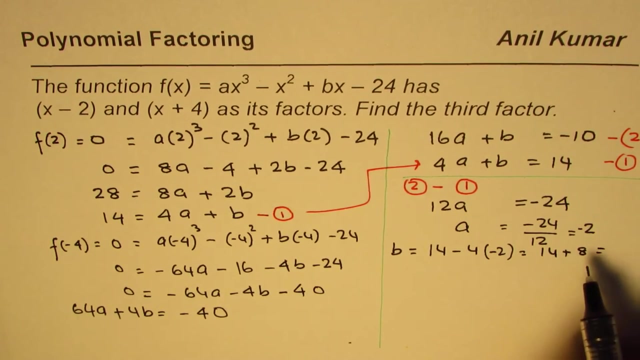 You can find the value of b by substituting a as minus 2.. So b will be equals to 14 minus 4 times a, which is minus 2, which is 14 minus, and minus is plus. plus 4 times 2 is 8, right, And that gives you the value of. 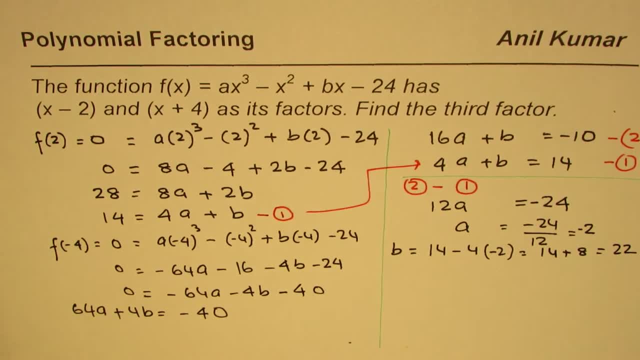 at 22,, right, Okay. So we'll soon need a calculator to further do our question, I think, Okay. So 14 plus 8 is 22.. So we get the value of b. So that gives us the polynomial, And the polynomial is f of x equals 2.. A is minus 2.. So we have minus 2 x cubed, minus x squared. 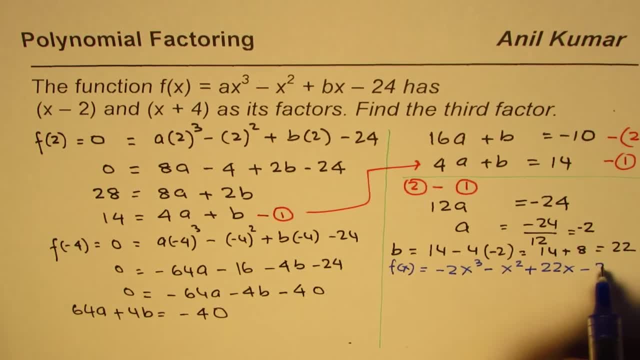 Plus 22 x minus 24, correct. So that is the polynomial for us. Now we need to get the third factor correct. We already know two of these factors. The different ways to find the third factor is that you could divide this by one factor. you get a quadratic equation And you know one of them is and find the factors for the other one to get the third factor. 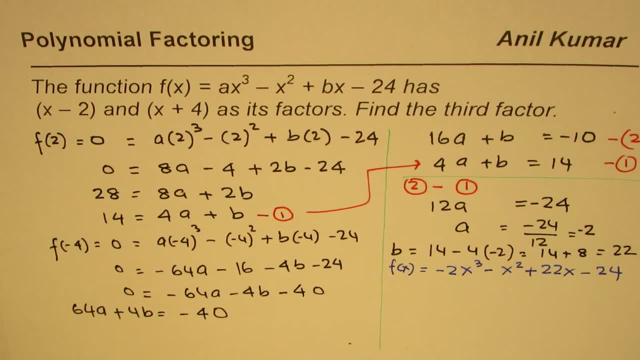 You get your result. So that should help you to get the third factor correct. So what I will do here is quickly, in this little space, divide it by the first factor. So we'll use the shortcut method to divide And let me show you here We'll write down these coefficients. These coefficients are- let's use a different ink- minus 2 for x cubed, minus 1 plus 2 for x squared. 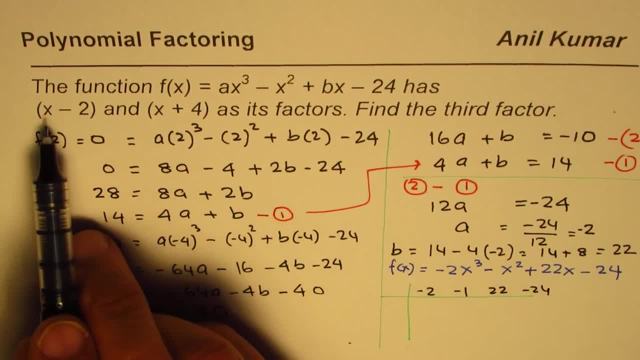 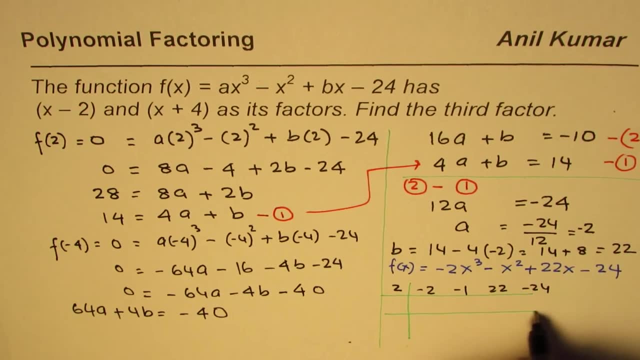 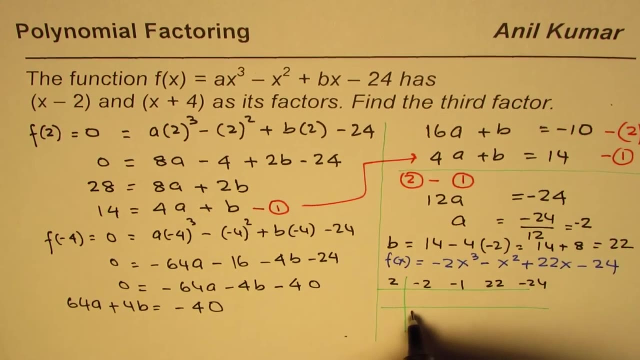 Plus 22, minus 24.. We are first dividing by x minus 2.. So we'll write 2 here. Now to divide. let me push this a bit here. We'll bring down 2.. I hope you know this division. Okay, So it is minus 2.. Multiply this by minus 2.. We get minus 4.. Add them up: minus 5.. Multiply, you get minus 10.. Add them up, you get 12.. 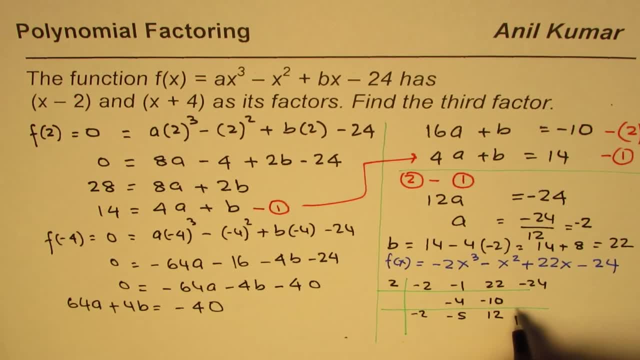 Multiply, you get 24.. Add them up, you get 0.. Correct, So that means the remainder is 0.. Indeed, this is a factor, But this gives you the quadratic equation which is minus. these are the coefficients right Minus 2x squared, minus 5x plus 12.. Now, if I divide this by the second factor, I get my result: Okay. 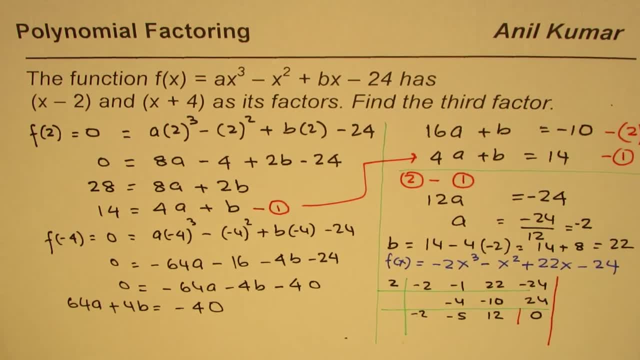 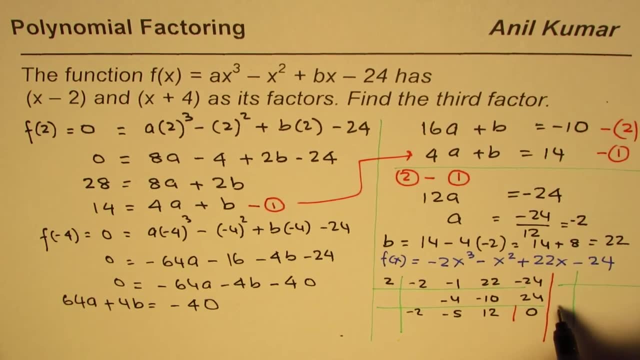 Running out of space, I'll just do it on this side, Okay. So let me use this space to do it shortcut. Okay, That's fine. What you can do is you can actually multiply these two and do long division and get your third factor. So here, these are my coefficients. So I'll write these coefficients here And once again divide. So we have minus 2,, minus 5, and 12. And this time we divide by 2.. 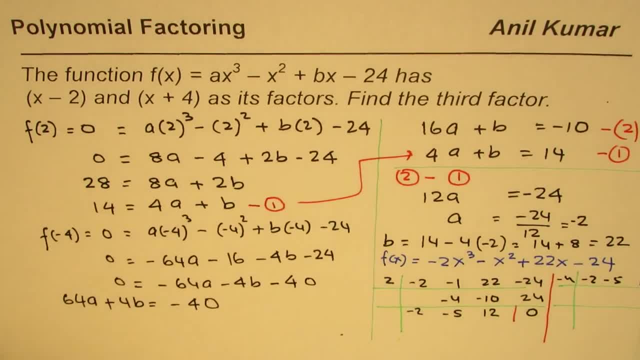 I'm dividing by minus 4.. Whatever makes this 0. That's the whole idea. In division we normally subtract, since I've taken minus 4.. What makes it 0?? I'm adding it up right. I'm not dividing by x plus 4, as we will do in long division. Okay, So this is synthetic division. So bring down this term minus 2 times with minus 4.. So it gives you 4 times 2 is 8 with positive sign, And then that gives you 3.. And when you multiply that with 3, you get 4.. 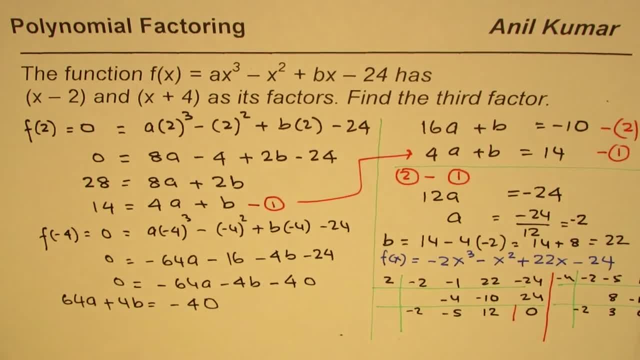 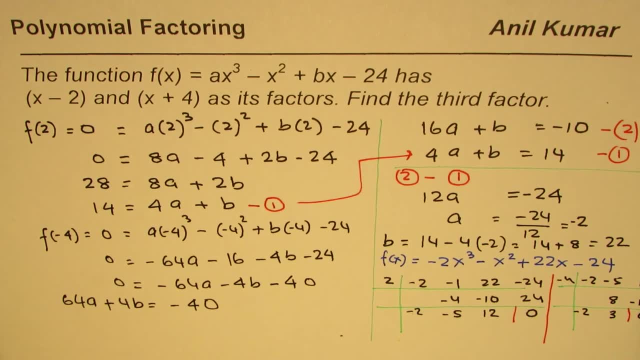 3,, you do get minus 12.. And the remainder, as expected, is 0. Correct, Remainder is Perfect. So there is your answer, which you can see right here. The answer is: these coefficients Correct For your quadratic, I mean for your linear function. Since this was quadratic, this is linear. So the third factor- let me write down the answer directly- is minus 2x plus 3.. Okay, 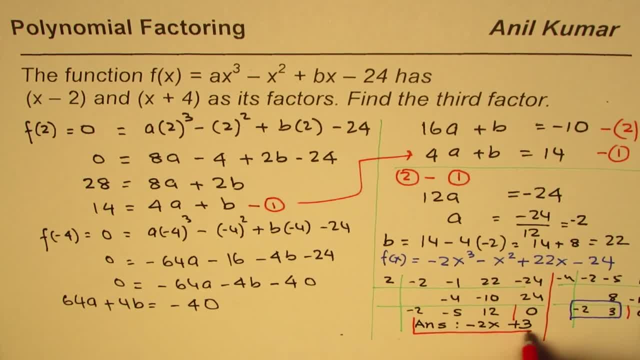 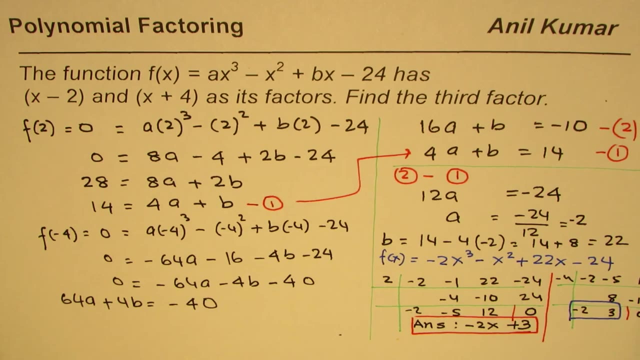 That is our factor. Okay, That's the answer And that's the third factor. Okay, Sorry for you know, just making it so tight with the area we have to work with anyway, But I hope the concept is clear to you. Let me go through this solution once again. We are given a polynomial in which we have two unknowns, a and b. So we need to find the coefficients of x cubed and that of x before finding the third factor.